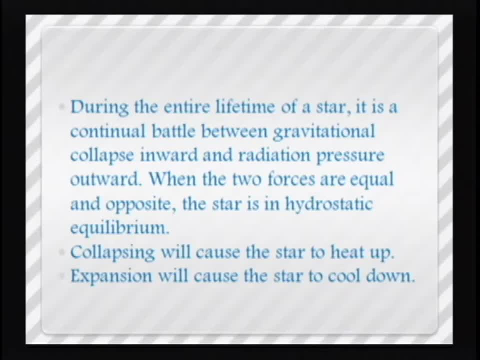 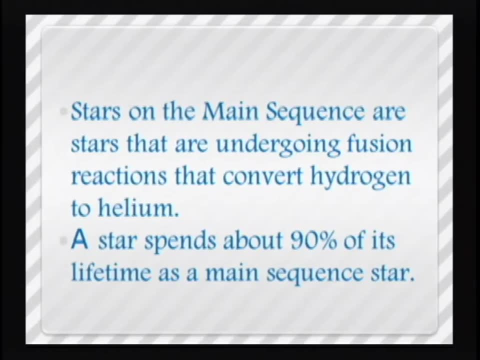 and contraction, But it's not a huge amount, not like what we're going to see as we start talking about the evolutionary sequence of these stars. So, as I said, those stars on the main sequence are undergoing that thermonuclear reaction. They are converting hydrogen into helium. 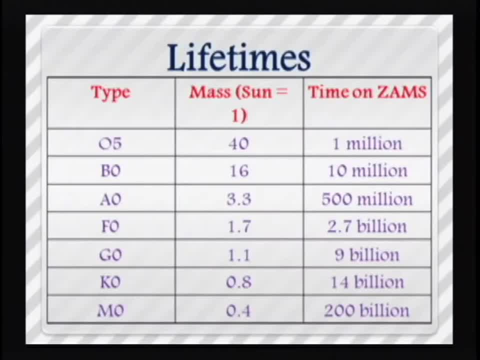 We've also said the star is going to spend 90% of its lifetime as a main sequence line. So what does that mean? And what temperature? or, excuse me, what temperatures? what times are we really talking about? Also, remember, guys, we talked about O, B, A, F, G, K and M. O. be a fine. 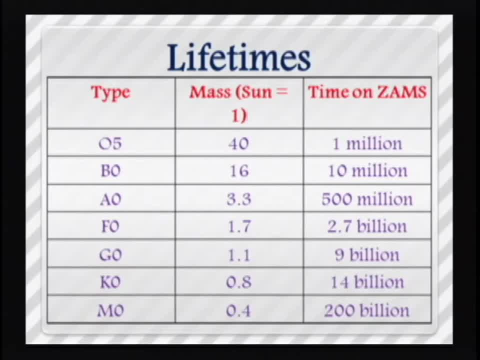 girl, kiss me. Or if you're a girl, O be a fine guy and kiss me, Okay, and so that gives you the order of the types or the spectral classifications, And so you can see on this chart I have lifetimes. 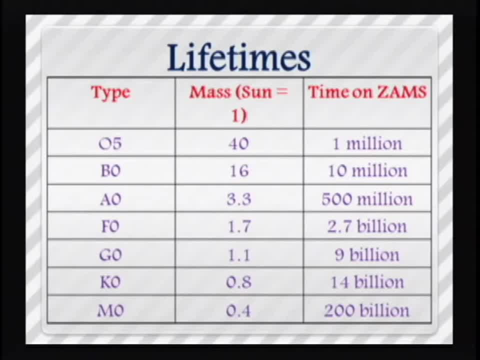 I have type, I have the mass and I have the time on this: 0AMS. What is that? Well, 0AMS stands for zero age main sequence. It's just another way that astronomers like to refer to that line as that main sequence line. 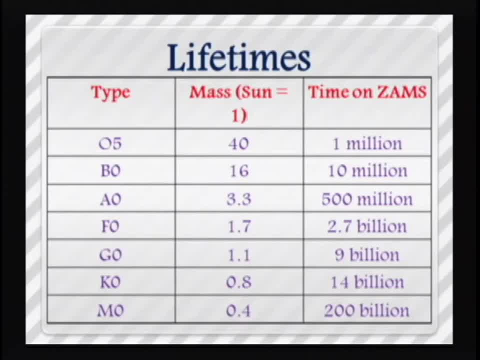 they put on, say, a zero age. So look, if I'm talking about a star, that's an O-type star. it's really really really very large, very hot. you know. its mass is at least 40 times the mass of 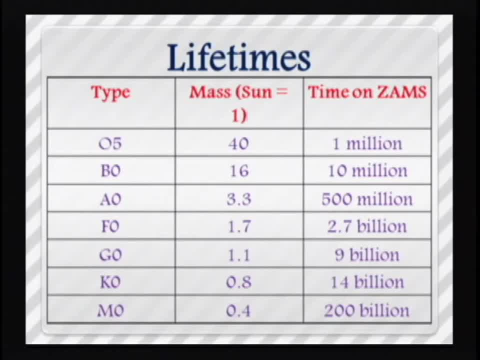 our sun, then notice the time that it's going to spend converting hydrogen to helium is only 1 million years. Now, guys, that's nothing more than a, you know, basically a snapshot, when we are talking about times relative to the universe. I mean, our universe has been around almost 14 billion years. You know that's. 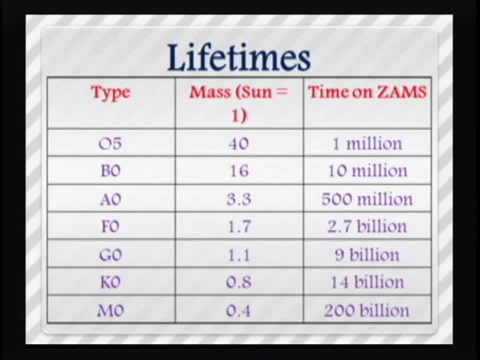 a tiny amount of time You know as that star, then if that O-type star was 50 times the mass of the sun, then it's even going to be less than a million years. I'm sure you guys have all heard the expression that the you know larger they are, the faster they fall. 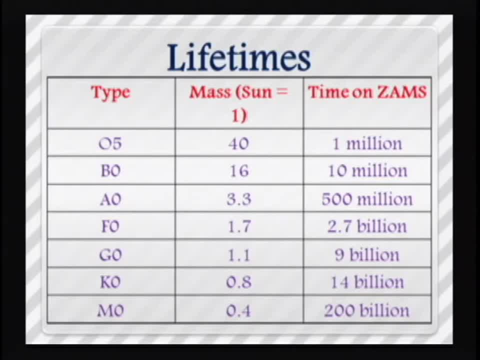 Well, that's definitely true when we talk about stars- B-type star 16 mass, so it's 16 times larger than the sun. It's going to be around about 10 million years. That's still not real long. I mean, 10 million years again is a tiny amount when we talk about 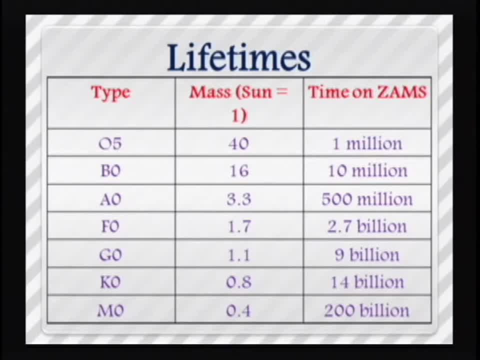 the age of the universe. An A0 star. it's about 3.3 times the mass of the sun. It's going to be here about 500 million and then it's going to start evolving off the main sequence line. Now, when I say evolve off the main sequence line, guys realize that it has nothing to. 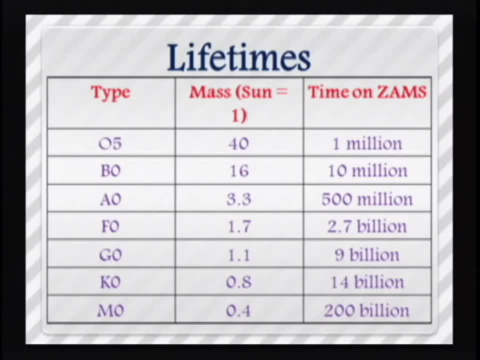 do with where that star is in the actual position in the sky. It just means that if I plot those two characteristics, looking at temperature or spectra classifications and looking at luminosity or brightness, then things are changing. They are no longer on that main. 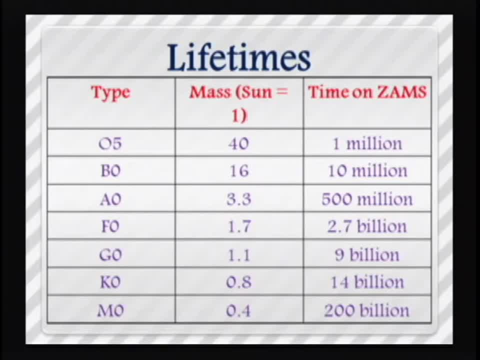 sequence line And then if I look at an F0, I'm looking at 1.7 million years. I'm looking at 1.7 million times the mass of the sun. Notice how long it's going to spend on the main sequence. 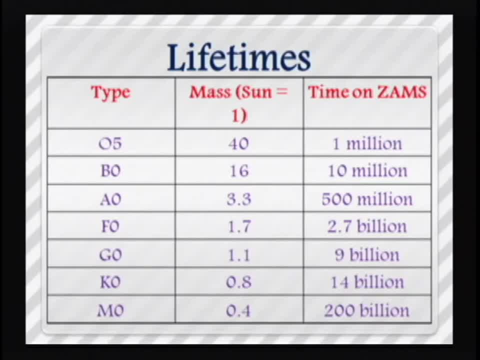 line 2.7 billion years- And yes, that is a billion with a B. So I've gone from 3.3 times the mass of our sun to 1.7 times the mass of our sun And I've increased the time. 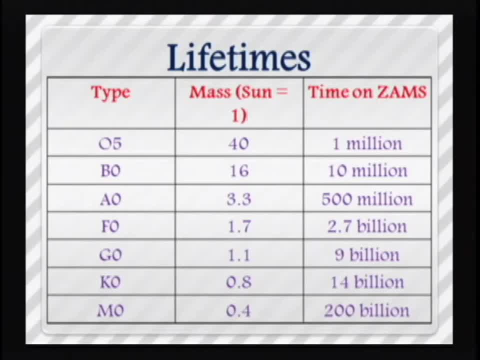 on the main sequence from 500 million years to about 2.7 billion years If I go down to a G-type star, G0, so it's a 1.1.. Notice that that's 9 billion. Remember we're a. 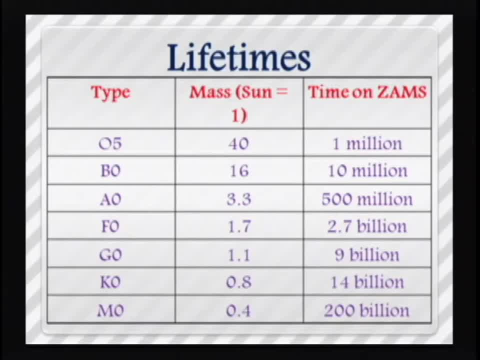 G2 star. so we're basically our mass and we're going to spend right around 10 billion years on the main sequence line. I get to those K0 stars. It's about 80% the size of our sun. Notice, it's going to be on there for 14 billion. 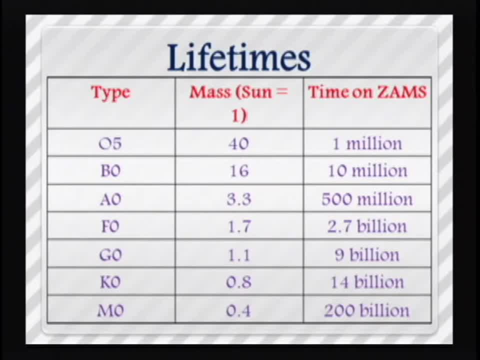 So we really haven't been around quite long enough to see a K0 star evolve off of the main sequence line. So you're down into that red dwarf region, an M0, about 40% the size of our sun, 200 billion years. Well guys, like I said, we've only been around, not quite. 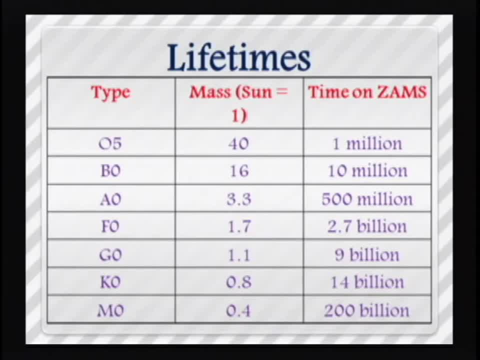 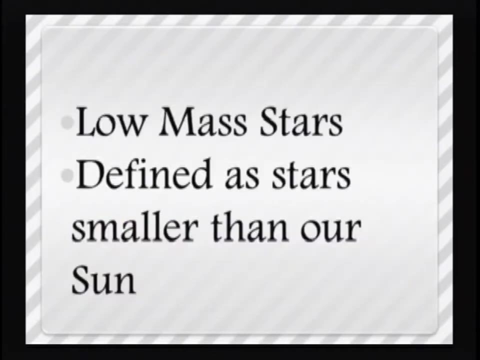 14 billion years And these lifetimes on the main sequence line for these red dwarfs are in the orders of 200 billion. We haven't even approached being around long enough to see one of those red dwarfs cool off and fade away. So, like I said, low mass stars are simply defined as stars that are. 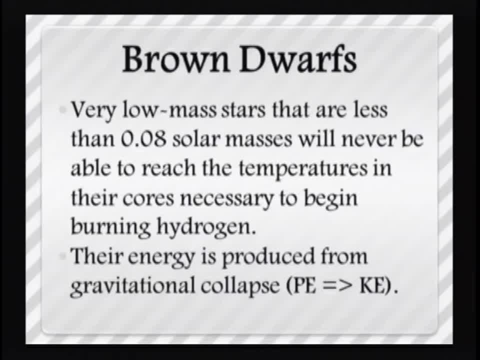 certainly smaller than our sun. And then I've alluded to these brown dwarfs, but want to go ahead and give you a definition at this point- And they're very low mass stars- And again when I say very, I mean really low mass- that are less than about 0.08 solar masses. 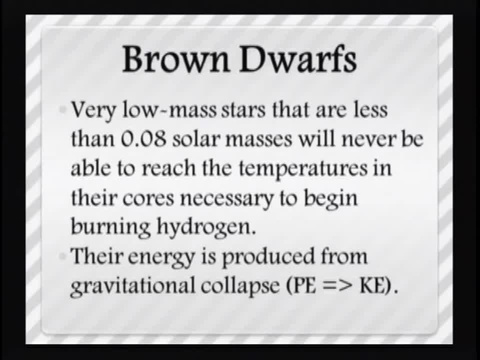 they're never going to be able to reach the temperatures in their core that's going to be required to convert hydrogen into helium, And so they've got to. then they are brown dwarf stars. then there's got to be some other mechanism inside there that's providing the 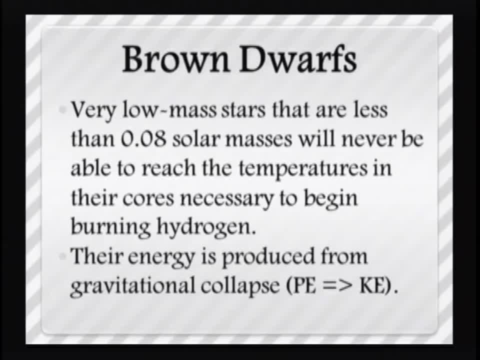 energy for them to go ahead and be seen to go ahead and shine, And we think that that's probably from gravitational collapse. Think back when you're fourth or fifth or sixth grade and you talked about kinetic energy as energy of motion and potential energy as 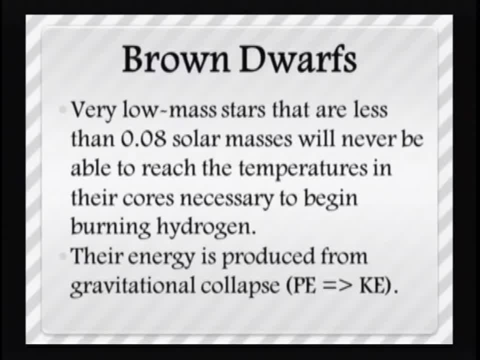 stored energy. Well, guys, we're doing the same kind of potential and kinetic here. You go ahead and you compress or collapse that star And as that material is going from an area of higher potential to a lower potential, then I get energy converted into kinetic. 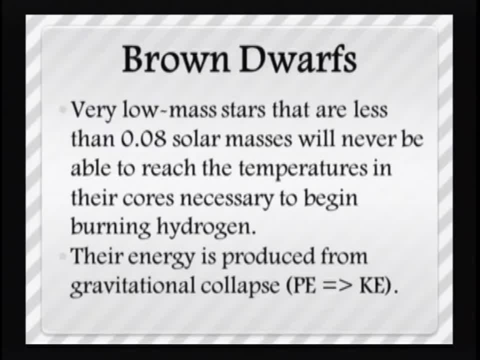 Remember the law of conservation of mass and energy. Energy and mass can neither be created nor destroyed. It can only change forms, And so you know this mechanism then, going from that potential to kinetic. that's going to be the same kind of potential and kinetic. 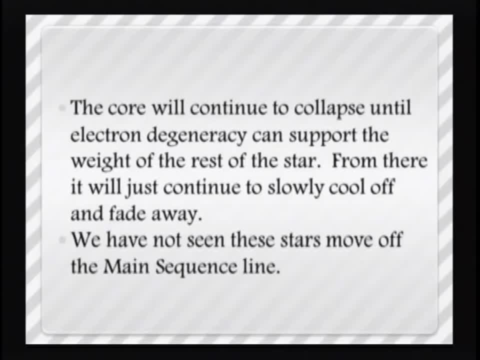 here. So that's what's causing those stars to shine. The star is going to go ahead and continue to collapse until we get to something called electron degeneracy, And that's going to support the weight of the rest of the star And then, like I said, it's just going to basically. 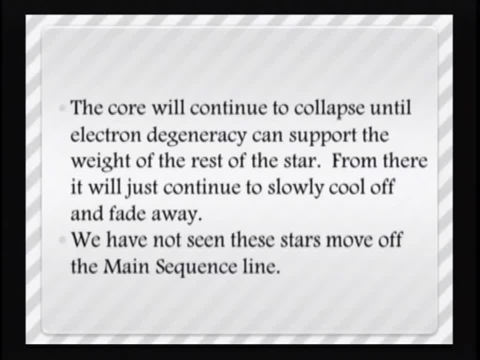 slowly cool off and fade away. Now let's talk about what we mean by that electron degenerate star. That just means, guys, that I no longer have other kinds of particles that are going. everything has been converted into electrons, basically, and the electrons, which are negatively charged particles, the core will go ahead and collapse to. 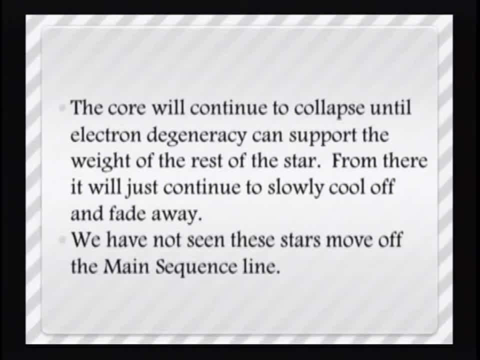 the point that everything is electrons and therefore I can't get any closer at that point. so the rest of the way to the star basically gets stopped from collapsing anymore on the core, because the core is made up of electrons and all those electrons are negatively charged and so you get a repulsion effect in. 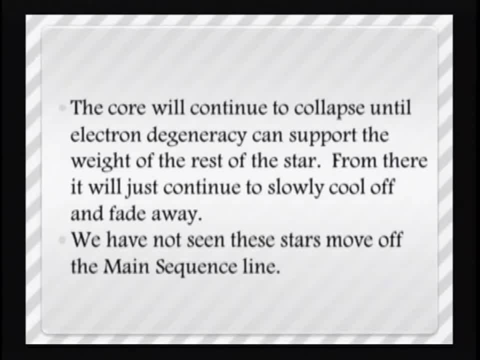 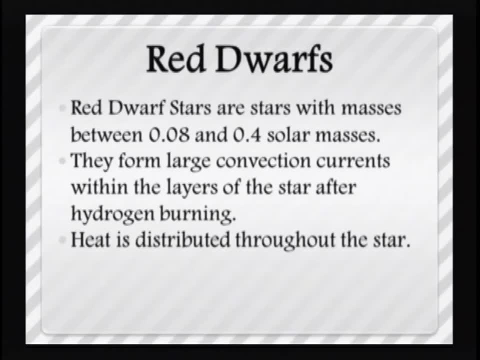 there and then, like I said, they're just going to slowly fade away these red dwarfs. then we've talked about a little bit. you know, now we're going back up and we will eventually get back up to the stars. that are very large, they go ahead. 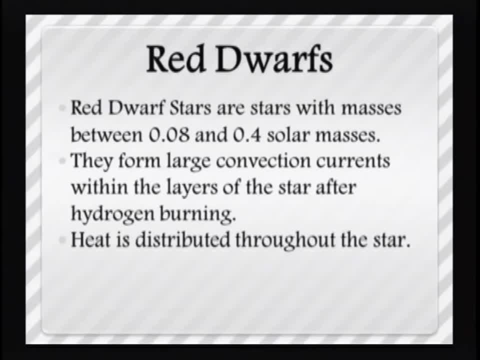 and form big convection currents within the layers of the stars, and so then you look at the heat that's being distributed to the star from those big convection currents. as compared to then, what was going within our Sun. you know the core and you had the 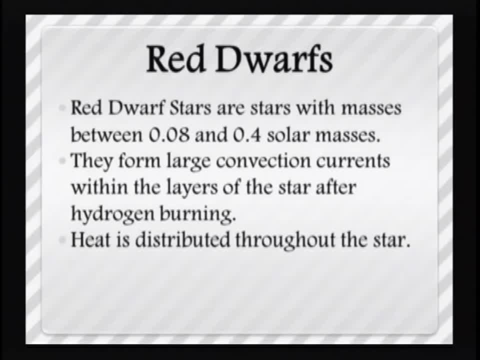 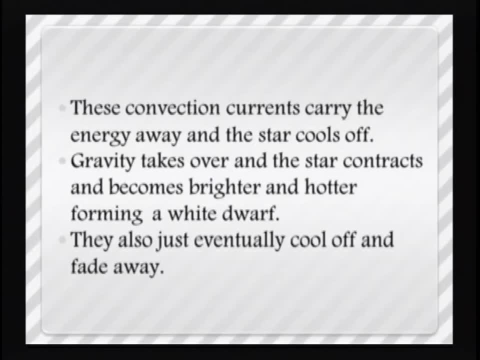 radiation zone, and then you had the big convection zone. well, these red dwarfs were never going to do that. they're never going to be able to set up those layers. okay, I said, these big convection currents are going ahead and take that energy away and the star goes ahead and gradually cools off. we think that then 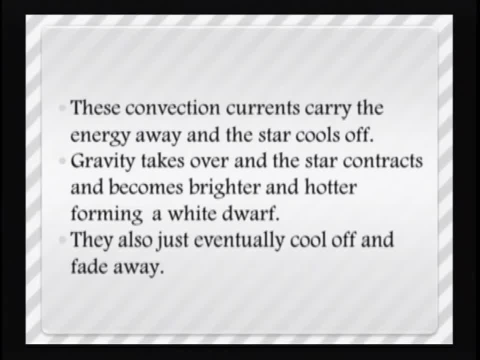 once that core is no longer producing energy, gravity, as with every other star, is going to take over, causes the star to go ahead and contract and that becomes a white dwarf. white dwarfs- remember, we're on the lower left hand. they are very bright, very hot. excuse me, they're very hot but they're. 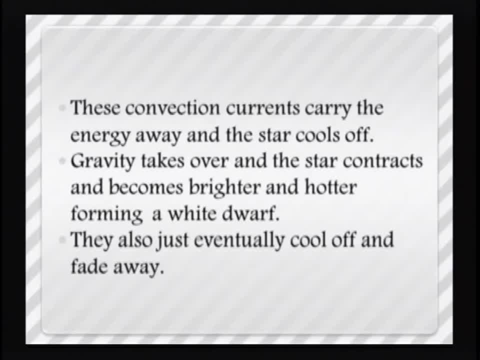 very dim, and so they're also going to do the same thing. they're eventually going to go ahead and cool off and fade away. so we know those smaller mass stars are ultimately going to cool off and fade away. the only difference is with what's going on within the star itself and the mechanism that finally then goes ahead. 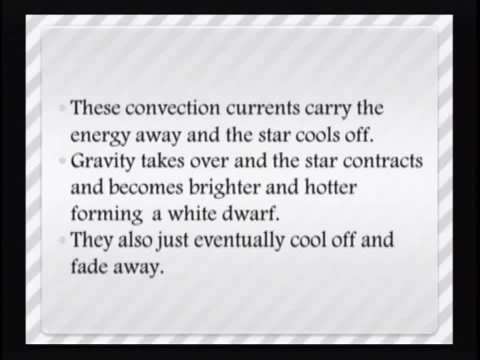 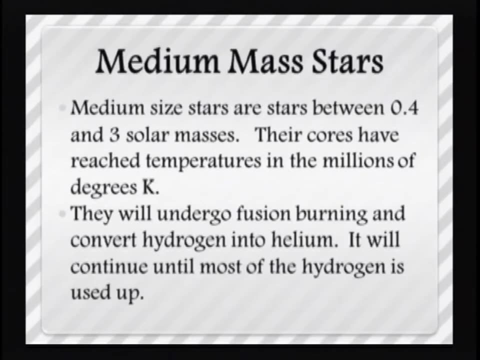 and provides that final energy, that then the star goes ahead and cools off and certainly, as I have said, and I will say again that mass makes that really big difference, and so mass determines what's going on inside that star. now, medium sized stars, or medium mass stars, as I showed you on that little table, or stars between about 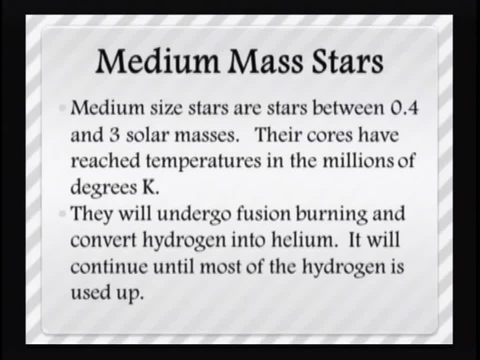 0.4 and 3 solar masses. really, these stars are very close to the Sun size and within the core they reach temperatures in the millions of degrees Kelvin. they, on the other hand, unlike the brown dwarfs and the red dwarfs, are going to undergo some 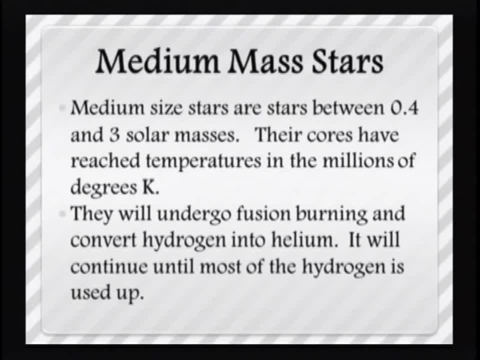 additional fission reactions and they're going to go ahead and convert hydrogen into helium and you know that's going to continue until you kind of run out of hydrogen, you have some helium left, and then we're going to find they go through the helium burning stage. so they're actually going to go through. 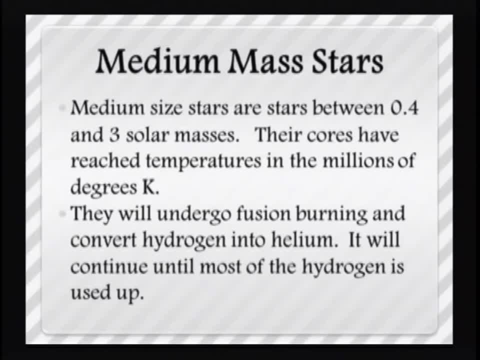 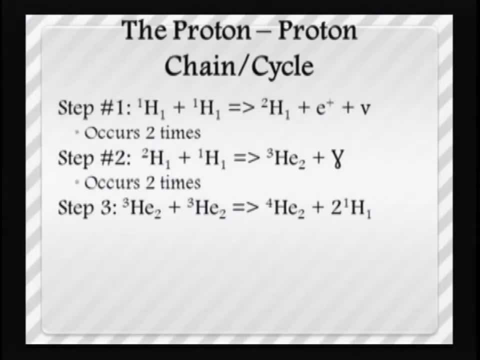 more stages within their core than what the brown dwarfs and the red dwarfs do. you've seen this before, you know. looking at that proton proton chain, same kind of thing that's going on the sun, so we're not going to worry about that too much. 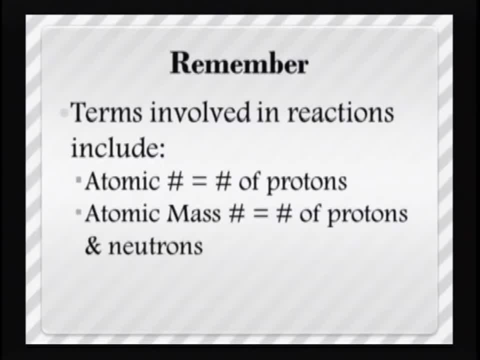 because you've seen it before and we've talked about it. just kind of want to remind you, as we go ahead and start talking about these stars and their evolutionary sequence, that atomic number is a number of protons. atomic mass number, number of protons plus neutrons. remember, guys, as we 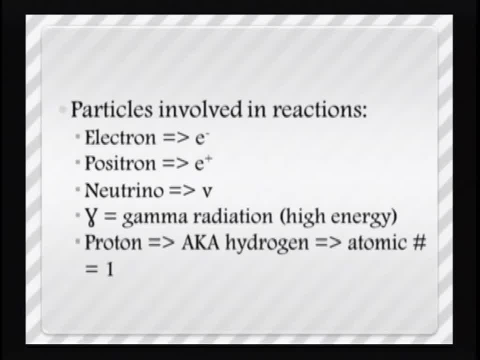 continue looking at these reactions. you have electrons. you have positrons, which are positive electrons. you have neutrinos, which are essentially massless, chargeless particles that go ahead and help carry away the hydrogen that's going to go through the neutron chain. so you're going to 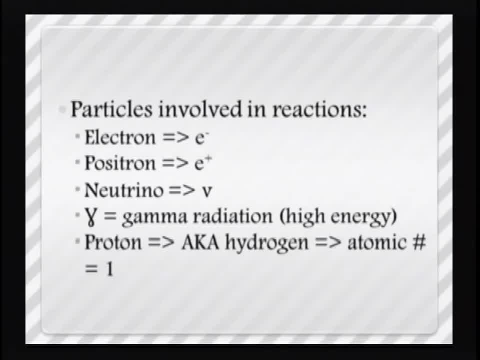 away all this, about 3% of the total amount of energy. We have gamma radiation, which is what you see, that really goes ahead and powers those stars, And that proton is also known as a hydrogen nucleus, which has an atomic number of one. All I'm doing is just 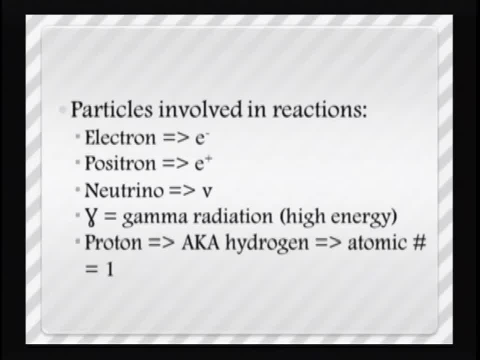 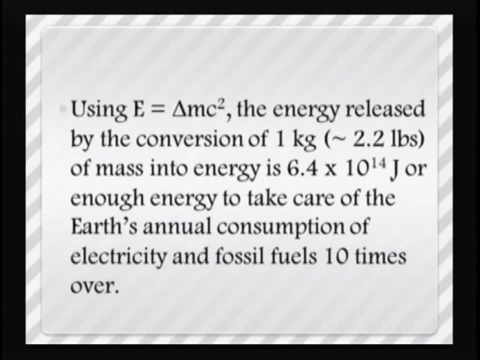 kind of reminding you some of these terms so that when we start talking about what's going on you can remember and refer to these. We've also talked about E equals MC squared, so I'm not going to go over that. We've also talked about this one. just again to remind. 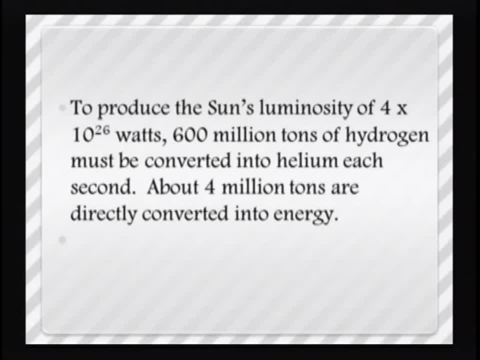 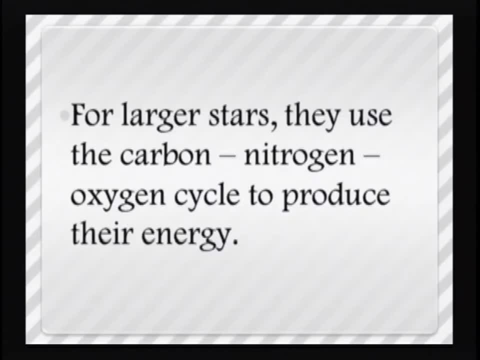 you how much energy these stars are using and how much mass they're having to convert into that energy according to Einstein's equation. Now, for larger stars they can't quite use that proton-proton chain. You know we have those two steps that produce the neutrinos. 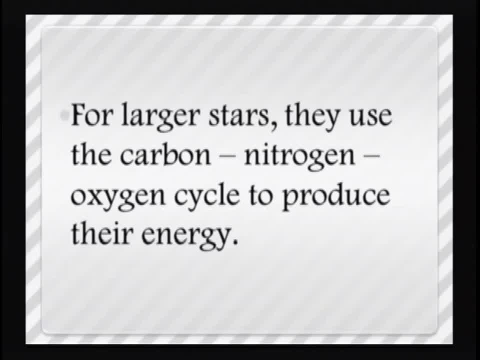 We have those two steps that go ahead and produce the gamma radiation, but that's not a enough to go ahead and fuel these really, really, really big stars. If any of you have children, think about you've got a kid out there that's playing football. He's a really 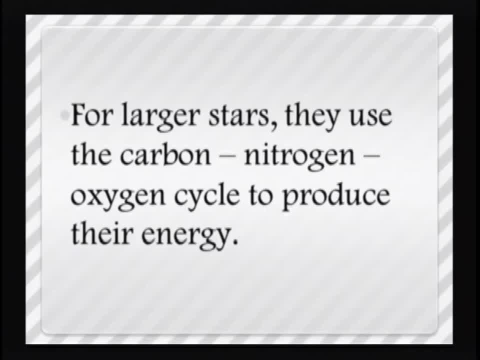 big stocky kid, You know there's a good chance that he's going to clean out your refrigerator. I mean, when my nephew was growing up and he would come up and visit me- and he's a pretty good-sized guy- I couldn't keep enough food in my refrigerator, you know. So they're. 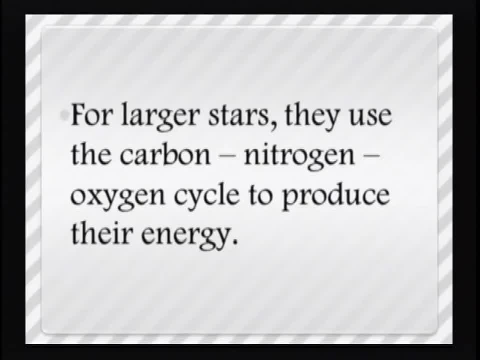 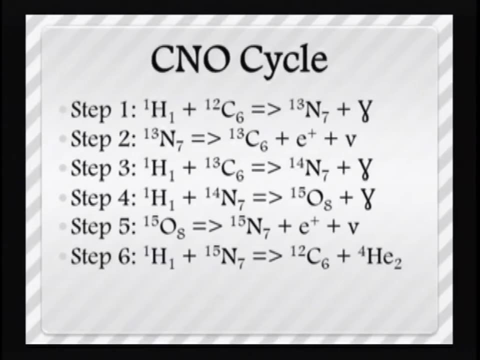 going to need lots and lots and lots of energy, No matter what size they are, they're simply using a tremendous amount of energy, And so we've got to come up with another mechanism to go ahead and be able to look at producing this energy, And so we do that with a carbon, nitrogen and oxygen cycle. So let's look. 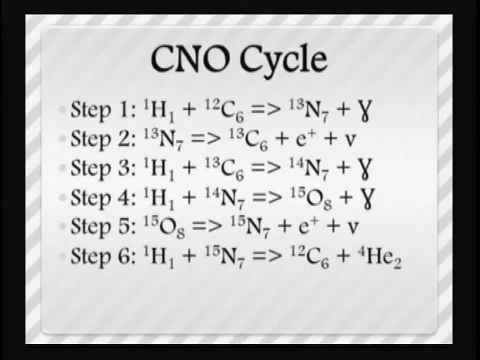 at these steps. We've already gone through that proton-proton, so a lot of these particles and those kinds of things should be familiar with you then. So we start with hydrogen now And we add that to carbon And carbon has six protons- six protons and six neutrons- And notice we're going to convert. 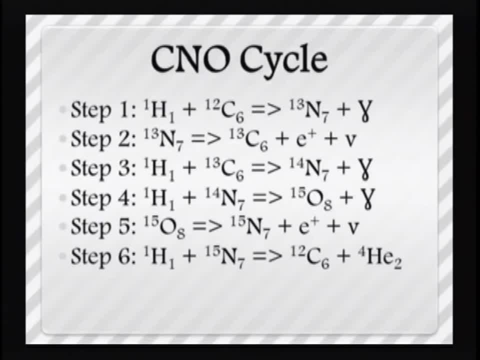 that into nitrogen-7.. So nitrogen-7 has seven protons and you can see there how many neutrons. But more importantly, we're getting gamma radiation given off. Remember that gamma radiation is nothing more than pure energy and that's going to help support that star. Then, in step, 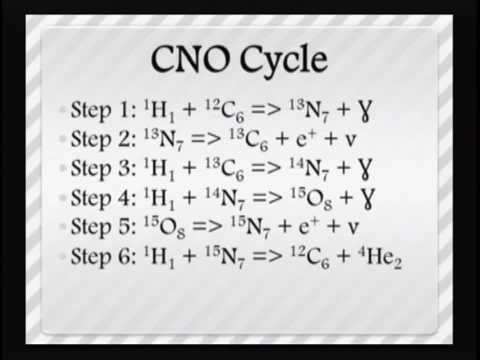 two. we take our nitrogen: It's unstable, So it immediately gives off a certain amount of energy. It's unstable, So we have a neutron given off, We have a positron given off And we have a neutrino given off. That neutrino, remember, is also energy, Not as much as what. 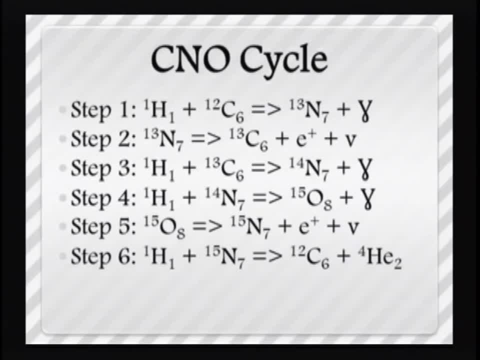 you're going to have in a gamma ray, but certainly it is energy. And remember that gammas are actual, just electromagnetic radiation, whereas a neutrino is an actual particle. Step three: you're going to take that hydrogen, that proton. This time you're going to react it with the 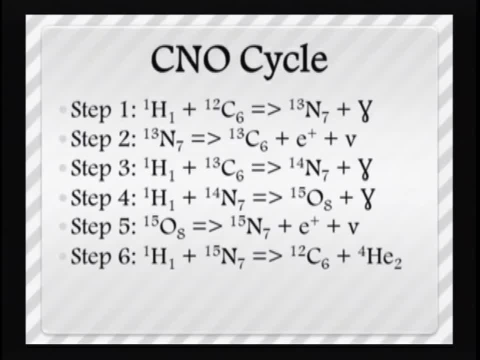 isotope, carbon-13.. You're going to produce nitrogen-14,, which means I now have seven protons and seven neutrons and I'm going to get another gamma radiation out, another gamma ray. Step four: take a hydrogen proton, add carbon-7 to it. excuse me, add nitrogen-7. 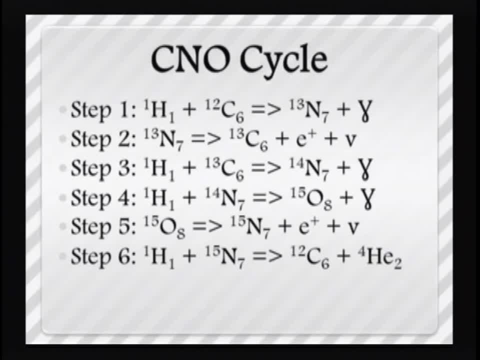 to it and you're going to form now oxygen Subtitles by the Amaraorg community. Okay, hence the name guys: carbon, nitrogen and oxygen. So you knew we had to have some oxygen eventually getting in there, And so I form oxygen-15.. Most of the oxygen that. 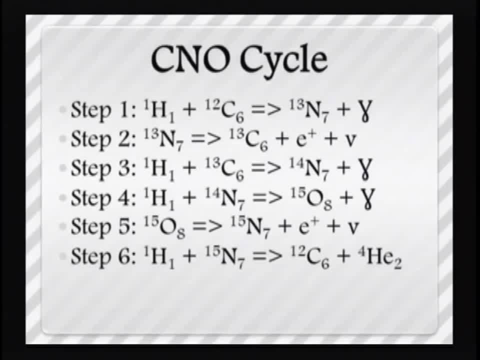 we see out, there is oxygen-16.. It has eight protons and eight neutrons. This has one less neutron, And so we find out that because of that one less neutron, it's unstable and it's going to go ahead and revert back to a more stable state. 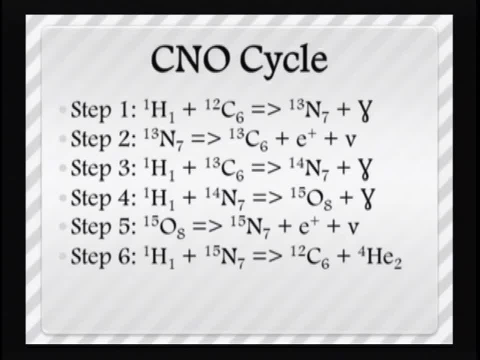 A more stable version, and that's what's going to happen in step five. Okay, So then you also notice that you have gamma radiation given off. Okay, So we've got that. oxygen-15 goes back down to nitrogen-15.. So I've lost a proton, I've gained a neutron. I give off. 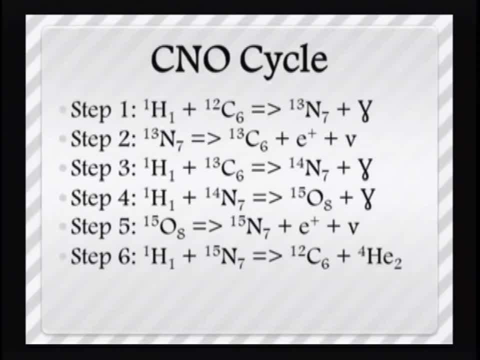 a positron and I give off another neutrino, And then step six doesn't give off any neutrons- Subtitles by the Amaraorg community, and I'm going to go ahead and start my cycle all the way over again. So there's a proton. 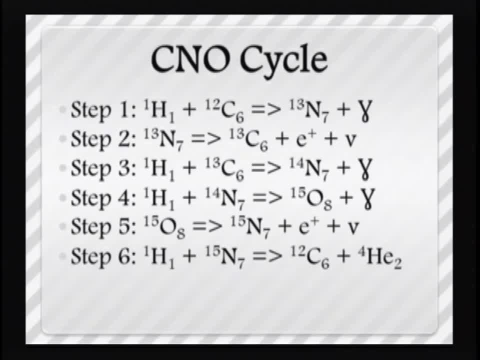 plus now I'm adding nitrogen-15.. That gets converted into carbon-12, which is certainly stable, plus then what's called an alpha particle. but an alpha particle is nothing more than a helium nucleus, And so it's that helium without the electrons, And, as I've said before, 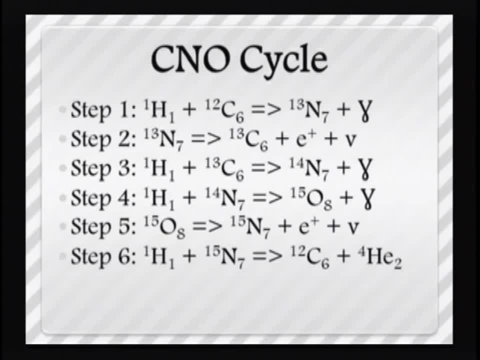 it's extremely stable. Subtitles by the Amaraorg community. I'm converting hydrogen into helium. It's just in those larger stars. within the core I have other materials besides just hydrogen and helium, And so I need those other materials to go ahead and give me enough energy that's produced in this cycle to power the star. 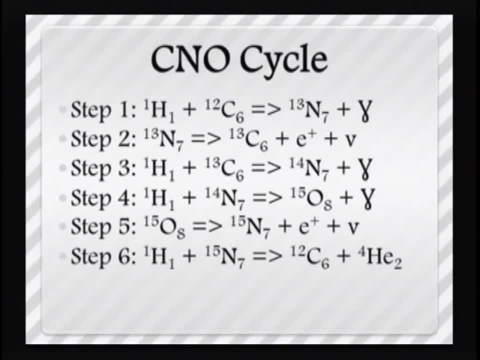 And so, if you look, you've got essentially five steps that are producing energy. Three steps are producing gamma radiation, and then two steps are producing neutrinos, And then step six, I get my carbon-12 again, which will allow me to start all over. So I'm again. 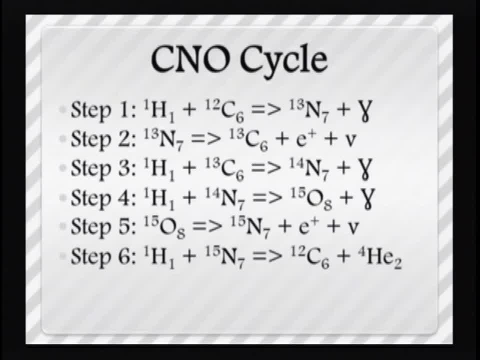 converting hydrogen into helium just through a different mechanism. Do I expect you to ever have memorized the proton-proton chain or the carbon-nitrogen-oxygen chain? No, But I do expect you, if you would see it again, to be able to use it and to understand what. 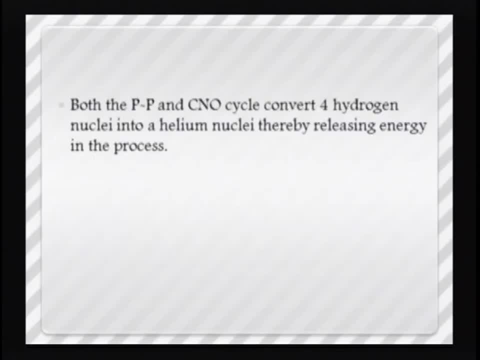 it's telling you Subtitles- by the Amaraorg community. Like I said, both the proton-proton and the carbon-nitrogen-oxygen cycle will go ahead and convert four hydrogen nuclides into helium. So, like I said, they're basically doing the. 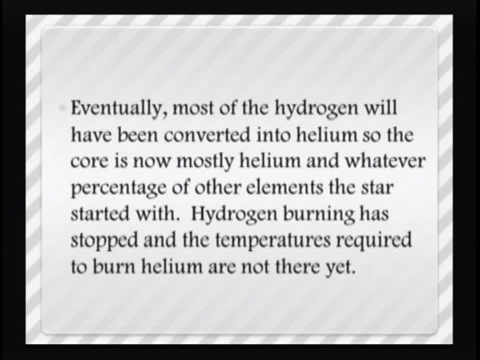 same thing, just through different mechanisms. Now, eventually, most of that hydrogen is going to have been converted into helium, And so when that happens, obviously things are going to start running down, And if we're talking about those really large stars, you're 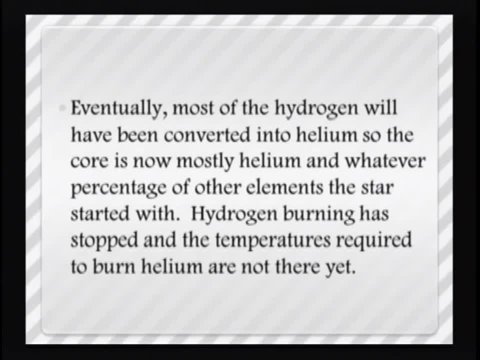 going to have lots of helium in the core and you're also going to have whatever other materials You might have had there to start with. So we're going to get this hydrogen burning. that's going to stop, But I haven't got the high temperatures yet required to go ahead, and 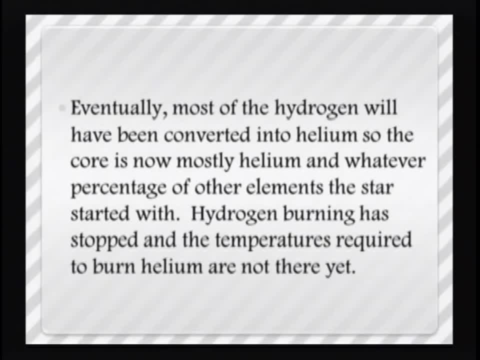 fuse helium. So what's going to happen if my hydrogen burning, that fusion process goes ahead and slows? I'm no longer in hydrostatic equilibrium. So therefore, the core itself is going to start contracting. Gravity is going to take over. Gravity is going to take. 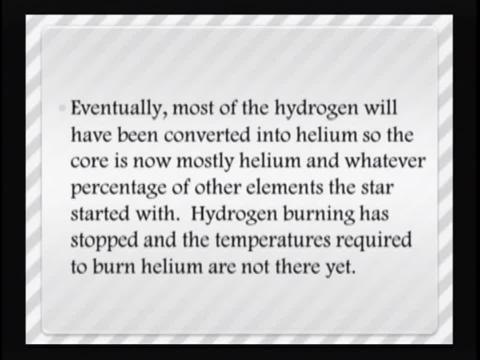 over and cause the core to contract. Well, guys, as the core contracts, the rest of the star recognizes that and kind of contracts along with it, And so that's why you're going to get kind of an instability region for just a little bit, until everything gets readjusted. 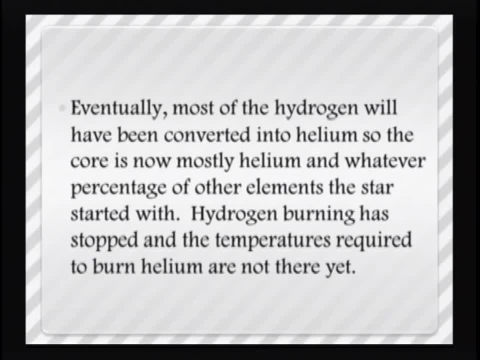 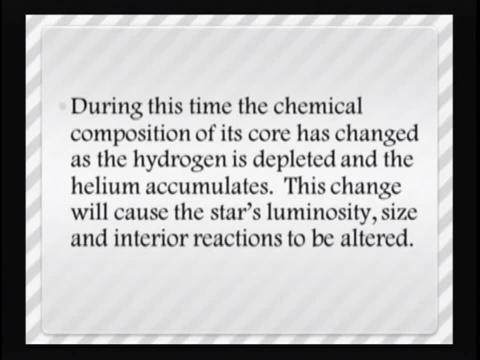 and that star can start burning helium. So, like I said, during this time that chemical composition has changed, you know, depending on what I have to start with, And so when that energy slows, or energy production slows or in some cases can almost stop, that 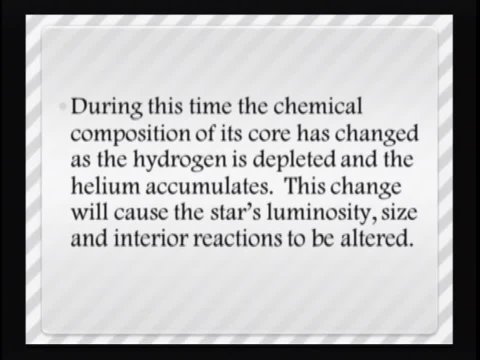 core is going to start collapsing, And when that core collapses then that's going to cause the star's luminosity size, everything that's going on in the interior, to go ahead and be altered, And that's then when we start having that star move off from the main sequence. 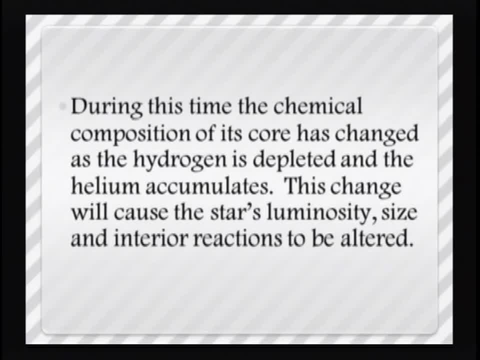 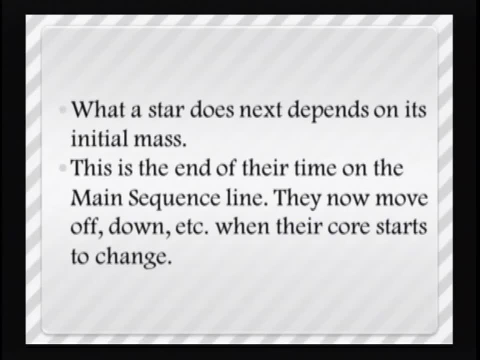 line to the various regions above that main sequence line. And, as we've talked, what a star does next is going to depend upon that initial mass. Mass is the single most important determining factor when you look at the evolutionary sequence of that star. Now gradually, then, as you're looking at that main sequence star, over time you are slowly- and I do mean slowly- running out of that hydrogen. So the rest of the core itself will go ahead and expand. Excuse me, The rest of the core will go ahead and expand. 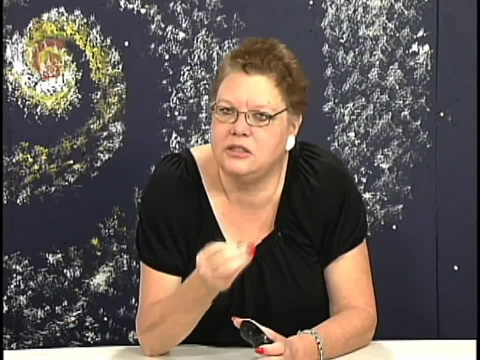 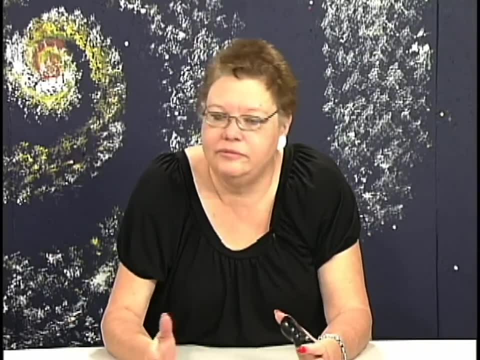 The rest of the core will go ahead and contract to allow for the fact that you are gradually slowing those reactions. And so if we look at our sun, we know our sun is brighter now than it was in the past. In the past it was about 70% of what we see now, And it's because 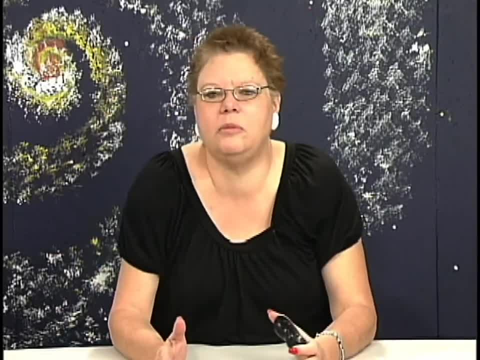 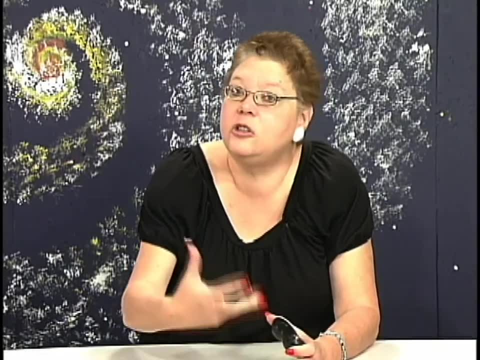 as the hydrogen is slowly, slowly stopping, you know, or at least slowing down. the rest of that core is going to respond to that. It's going to start condensing down a little bit to produce a little bit more of that energy that's given off, which is ultimately going. 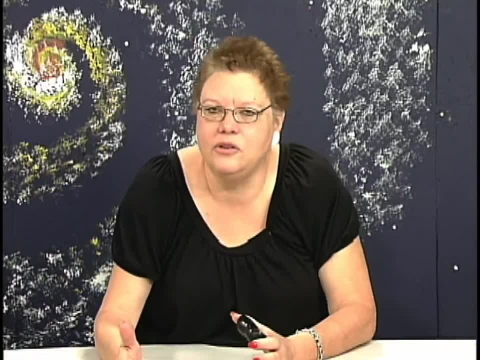 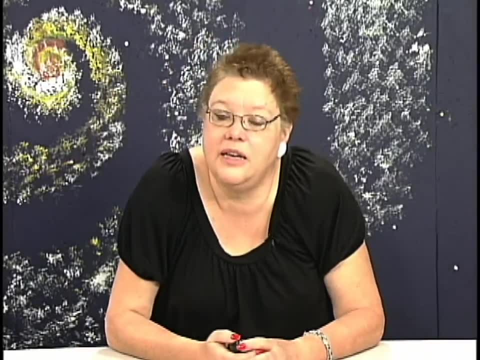 to cause the star to become a little bit brighter, And so you've got those kinds of reactions that are going on within the core itself that will gradually change over the period of time. that it's on the HR- excuse me, on the main sequence line, But still, guys, ultimately, 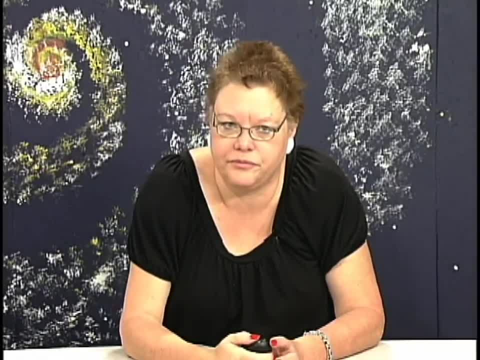 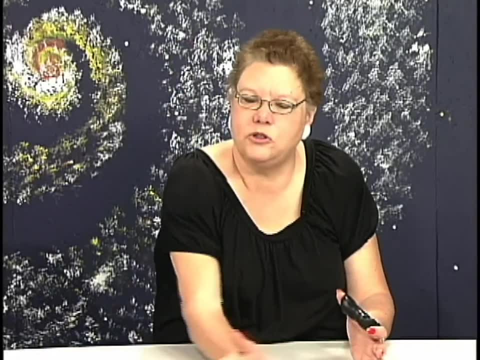 remember, the star on the main sequence line is converting hydrogen into helium. Now, once it stops converting hydrogen to helium, then, depending on its mass, we'll determine what's going on next. Okay, And that's what I want to talk about then. 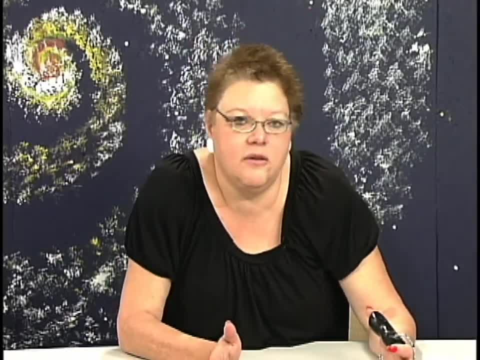 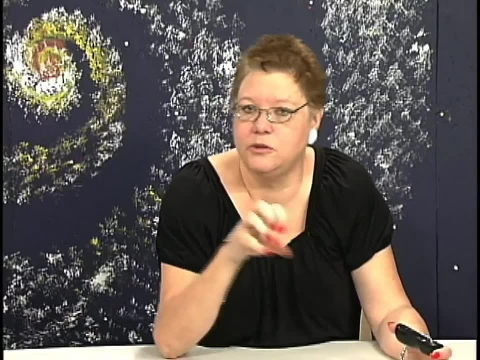 So what I want to talk about next is taking. okay, let's go back and let's look at these stars on the main sequence line. Let's break them up according to their mass. So we'll talk about these really massive stars, We'll talk about large stars, We'll talk about medium. 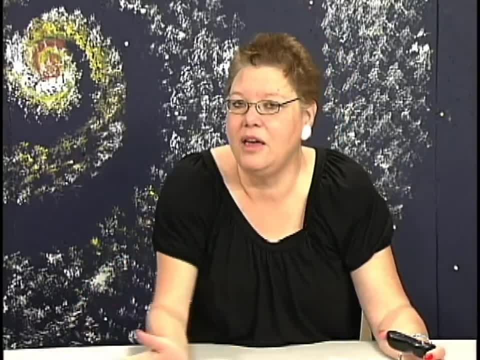 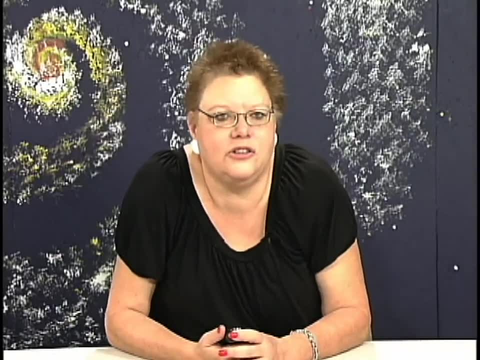 stars. We'll talk about the small stars. We'll talk about how they evolve off the main sequence line and how they ultimately end their life. And so, like I said, guys notice the last couple of sessions we haven't had any really cool pictures. That's because, when we come, 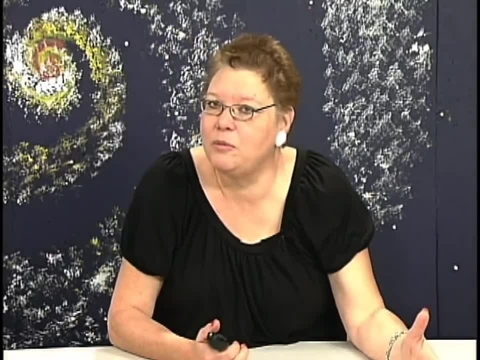 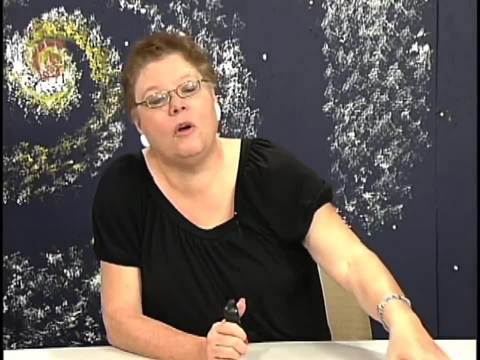 in next time. what I want to do is go back, start talking about a protostar And then no text. this time, guys, I just want to take you on a nice visual journey from the protostars all the way to black holes for those really, really, really large, massive stars. So make. 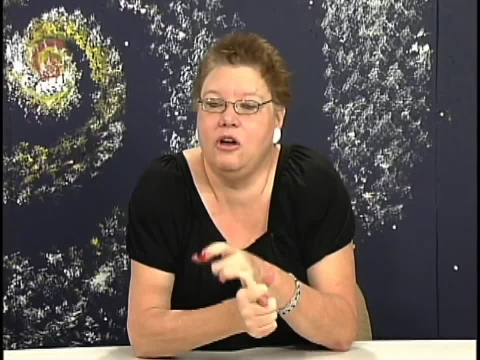 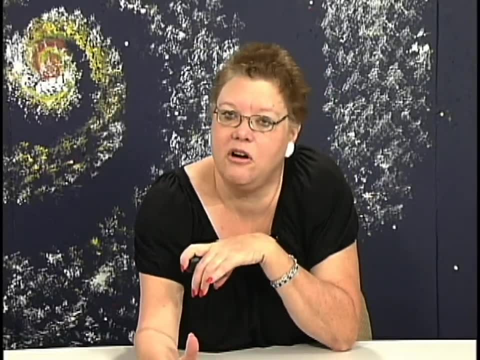 sure, between now and the next time you go ahead and go to Blackboard, pull off the sequences that I have for you on there that talk about the evolution of the stars, And I want that notes, those notes, basically to be in front of you as we go ahead and go through that. 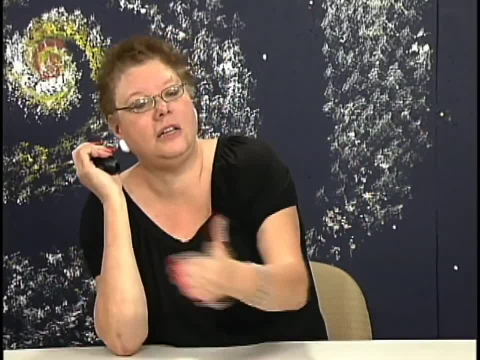 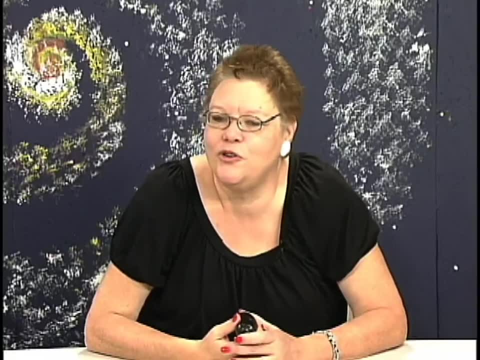 entire sequence from there, From a protostar to the end cycle of every one of those different mass stars. Okay, So with that guys, I'll plan on seeing you next time And be prepared for a journey out to the outer reaches of our solar system and beyond. So with that, talk to you later. Bye-bye.